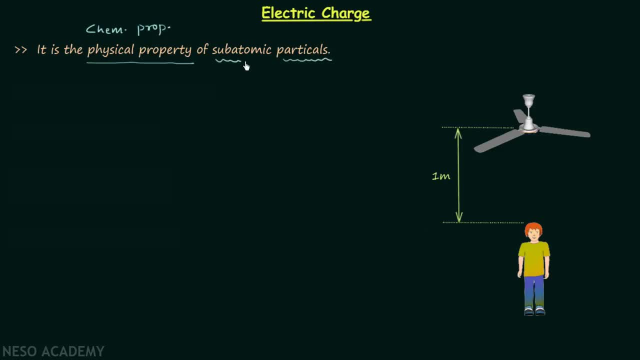 of particles which are subatomic in nature. Now, what do we mean by subatomic? As the name is suggesting, they are the particles which are smaller than the size of atom and they exist within the atom, And we are mainly talking about the two particles which are electrons and protons. 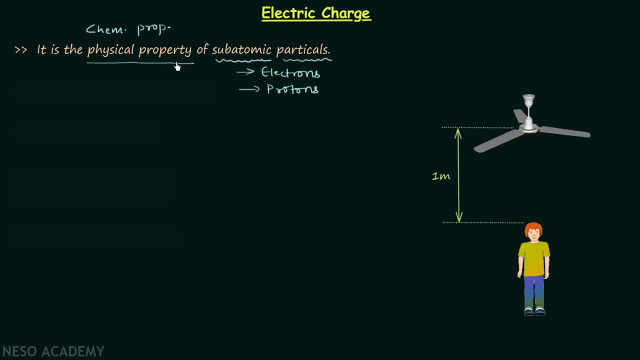 So we can say that an electric charge is the physical property of two subatomic particles: electrons and protons. So this is how we can define an electric charge. And now we will move on to the next point, And the next point will tell you. 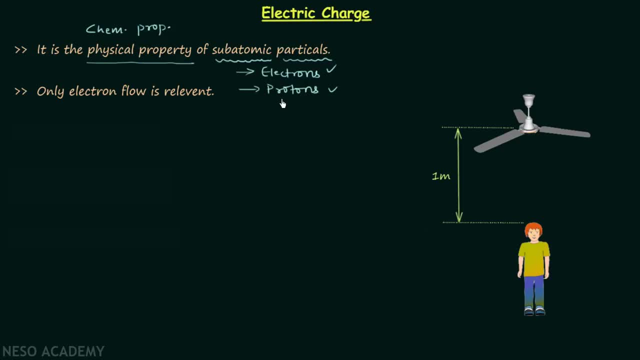 on what type of subatomic particle we need to focus in this particular course. In this particular course, we will mostly deal with the circuits in which only electron flow is relevant, So we will focus on the electron flow. This means we will focus on the flow of negative charge. 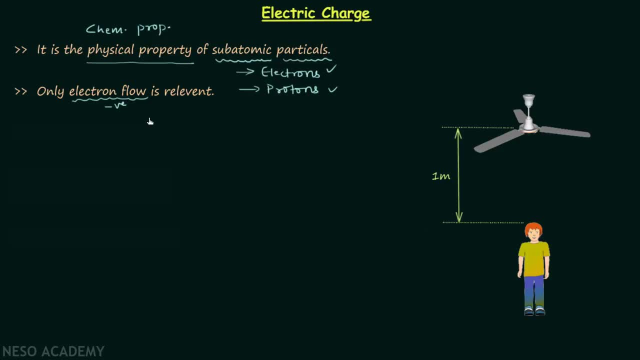 In many devices and circuits the flow of positive charge is on the finishing of positive charges and the flow of negative charges on. the winning issue Thereforeist just also relevant. like in case of semiconductor devices, the flow of positive charge is also relevant along with the negative charge flow, but there the positive charge is due to the presence. 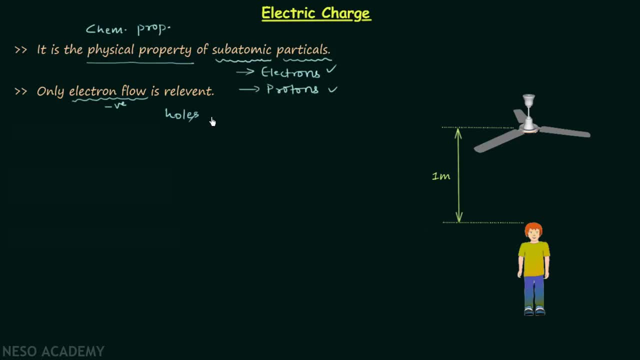 of holes. but in case of network theory, we don't have to worry about holes because holes are not present inside the metals. holes are present inside the semiconductors and they are not present inside the metals and therefore in network theory the positive charge will be due to protons. 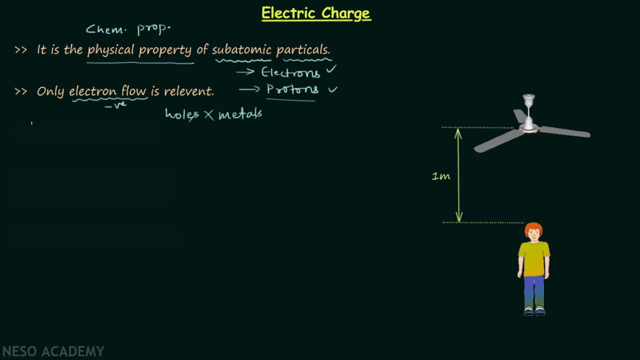 so this is all for the second point, and now we will move to the third point, in which we will talk about quantization of charge. by quantization of charge, we mean charge can move in the same way as the charge can move in the same way as the charge can move in the 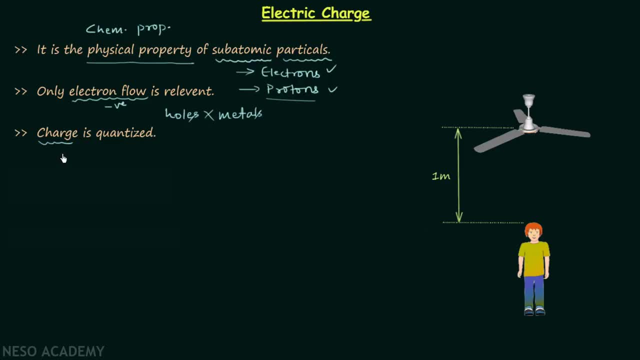 multiple interest levels. and here one of the things important is that the charge cannot exist in an arbitrary manner. this means you cannot have one by two E as the charge or 3 by 2 E as the charge. charge cannot exist like this, because charge is quantized. by quantization of charge we mean charge. 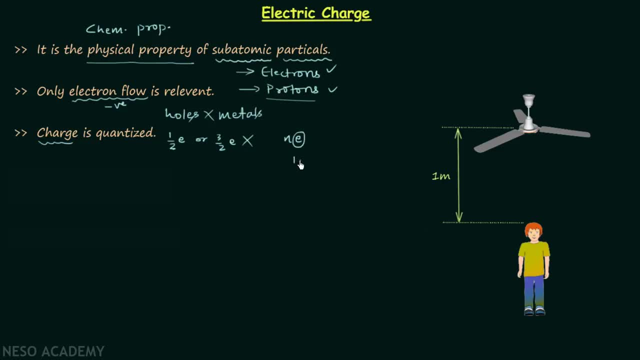 the elementary charge and E is equal to 1.6 multiplied to 10, raised to power minus 19 Coulomb. So we can say that the elementary charge is like the smallest packet of the charge and we cannot divide this packet further. Therefore, 1 by 2 E is not possible because this: 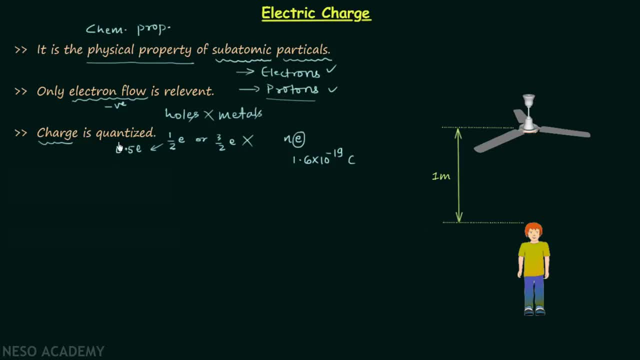 is equal to 0.5 E and in this case we are dividing the packet into two equal parts, which is not possible. Similarly, 3 by 2 E is also not possible, because this is equal to 1.5 E and we can write: 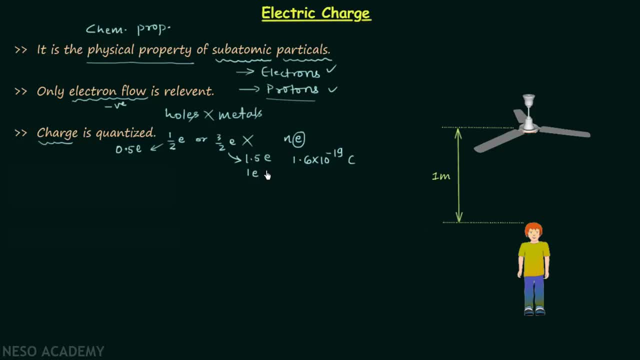 1.5 E equal to 1 E plus 0.5 E. This part is okay, but this part is not allowed, So we can have only integral multiple of E. This means the charge will always be equal to n times E, where n is an integer and the charge on E is equal to 1.6 multiplied to 10, raised to power minus. 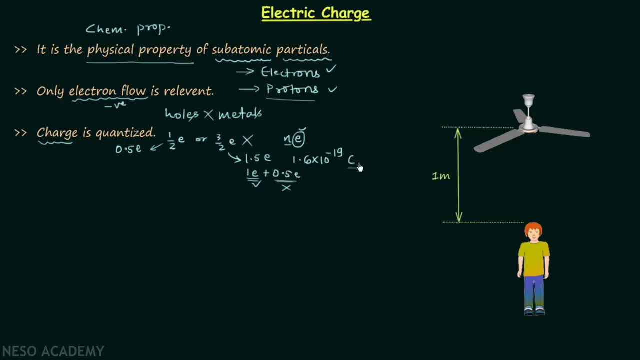 19 Coulomb. Now, what is Coulomb? Coulomb is the SI unit of the charge and it is named after French physicist Charles Coulomb. Coulomb is the SI unit of the charge and it is named after French physicist Charles Coulomb. 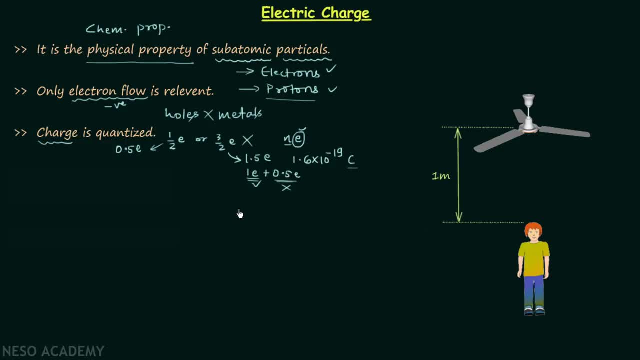 The charge can be of two types: the positive charge and the negative charge. Electrons have the negative charge and protons have the positive charge. Charge of one electron is equal to the elementary charge with negative sign. because, I told you, electrons have the negative charge. This means electrons will have charge equal to minus 1.6. 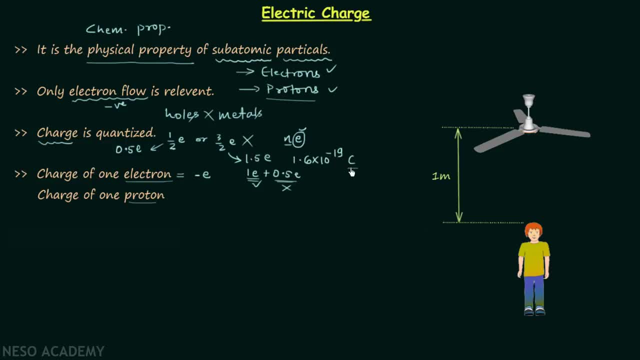 multiplied to 10, raised to power, –19 Coulomb. Similarly, charge of one proton is equal to plus E. this makes the charge equal to plus 1.6 multiplied to 10, raised to power minus 19 Coulomb. Now we will move on to the last point, which is an important point. This point is not at all important. 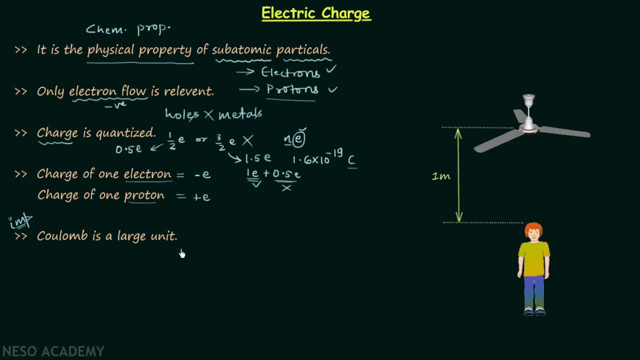 for your exam. this is important if you want to have good knowledge. according to this point, coulomb is a very large unit. this point is very straightforward: coulomb is a very large unit, but now we will understand this point. or you can say: now we will feel this point, why coulomb is? 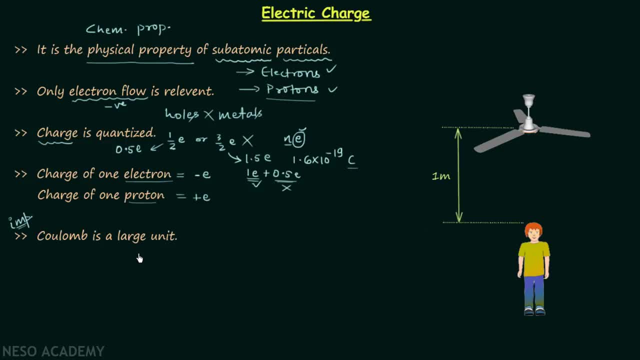 a very large unit by the help of two different examples. in the first example you can see the arrangement. we are having one ceiling fan and one boy is standing just below the ceiling fan, and the distance between the ceiling fan and the boy is equal to one meter. and now we will put one coulomb. 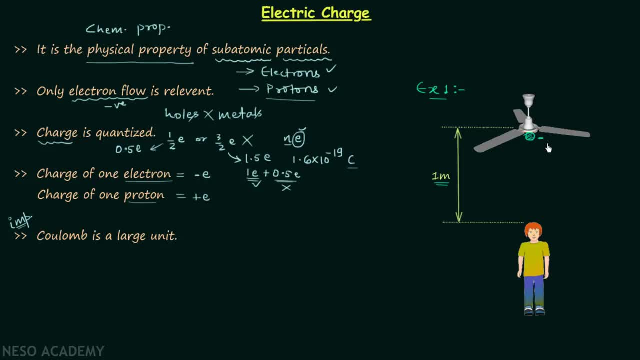 charge on the fan and the charge is negative charge. so we have minus one coulomb charge on the fan and we will do the same thing with the boy as well. we will put minus one coulomb charge on the head of the boy. now this boy looks very calm and he is enjoying his time. but according to 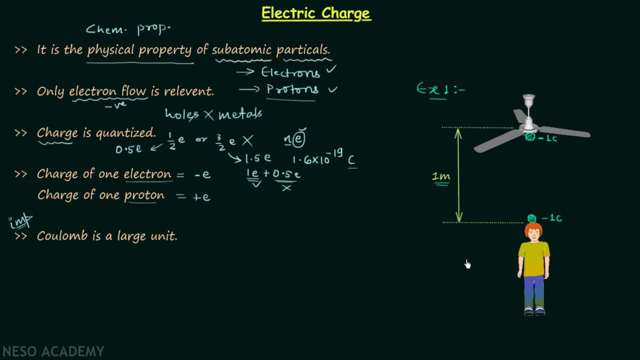 me he should be running because he is going to experience a very large amount of force. He will experience the force because we know when two similar charges are placed near, they will repel each other and therefore there will be a force of repulsion, and this force of repulsion will be equal to 9 multiplied. 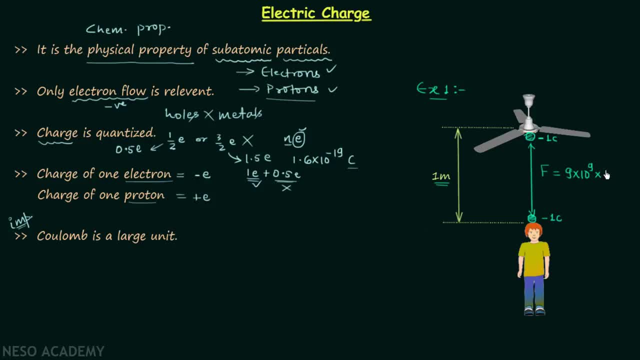 to 10. raised to power: 9 multiplied to the first charge, multiplied to the second charge, divided by the square of the distance between the two charges- and we are writing this using the Coulomb's law- and q1 is equal to minus 1 Coulomb. 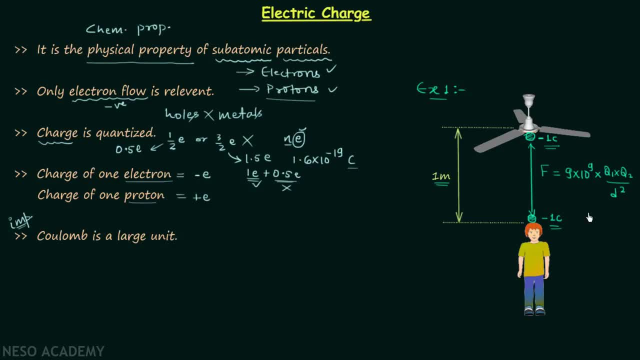 q2 is equal to minus 1 Coulomb and distance d is equal to 1 meter. So when you solve this you will get: the force of repulsion is equal to 9 multiplied to 10, raised to power, 9, Newton. 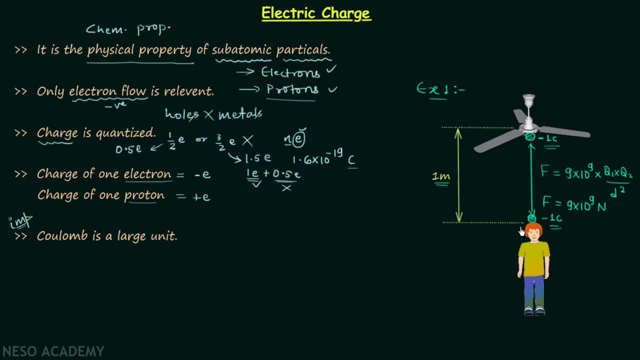 So this boy will feel a downward force equal to 9 multiplied to 10, raised to power, 9 Newton, and this force is equal to 9 billion Newton's. And we know 1 Newton is approximately equal to 100 grams. This makes 9 billion Newton approximately equal to 900 million kilograms. 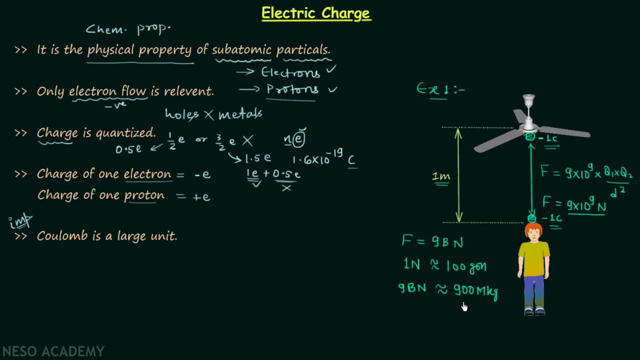 So this boy will feel the weight equal to 900 million kilograms on his head. So now you can have the feeling that how large is the force of repulsion? Now there is another example, and this example is the homework for you. In this example, you need to tell me how many electrons are there on the head of this boy. 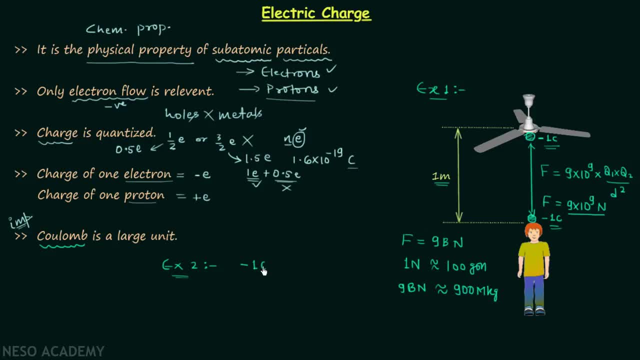 We are having the total charge equal to minus 1 Coulomb on the head of this boy and, corresponding to this charge, you need to tell me the total number of electrons. So this is your homework problem. So once you have the answer, post it in comment section. and when you have the correct answer, 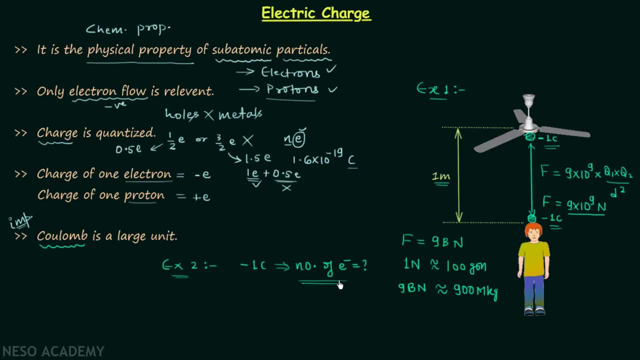 you will find a very large number of electrons are required to constitute 1 Coulomb charge. So this is all for this lecture. If you have any doubt, you may ask in the comment section. I will end this lecture here. See you in the next one. Bye-bye, Bye-bye.